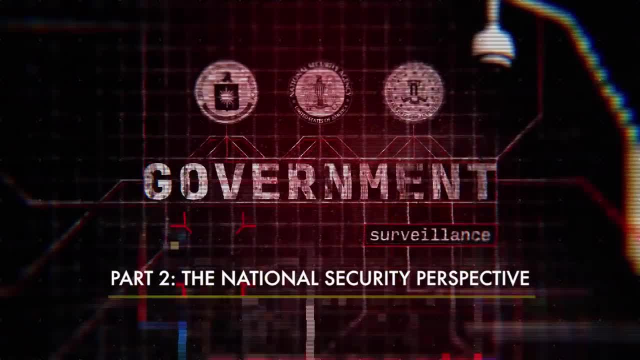 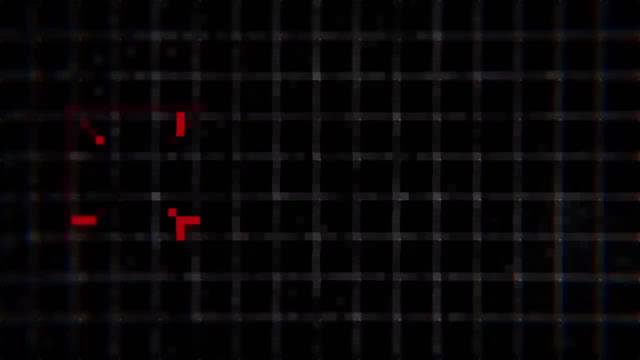 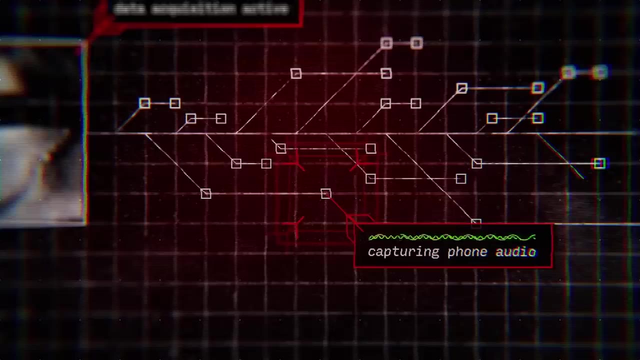 I think the other thing that's important in this debate- and it often gets confused- is people hear about collection of electronic information and they automatically assume that means the government's collecting an email, the government's recording my phone call, my conversation, A lot of the Snowden debate. 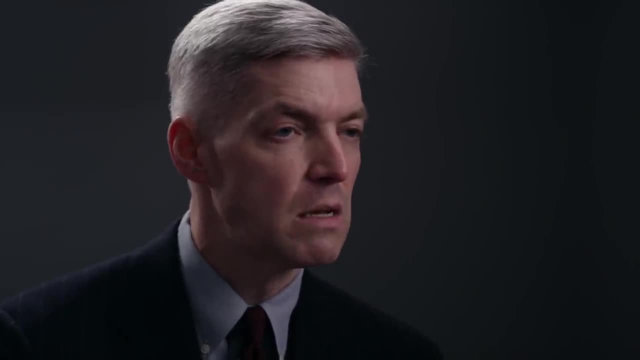 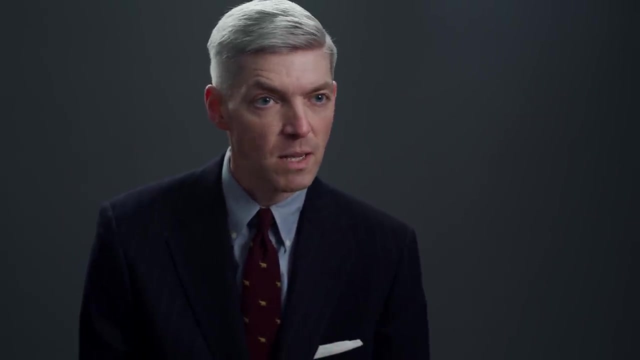 had nothing to do with that. It was simply metadata, which is the equivalent of the address on an envelope. It doesn't tell you what's inside the envelope. it tells you that someone sent me a letter or the header of an email, the to from. 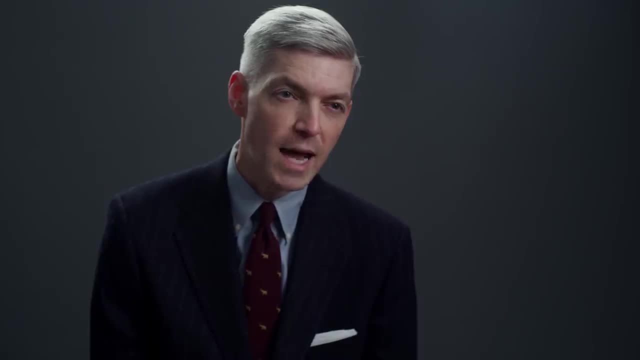 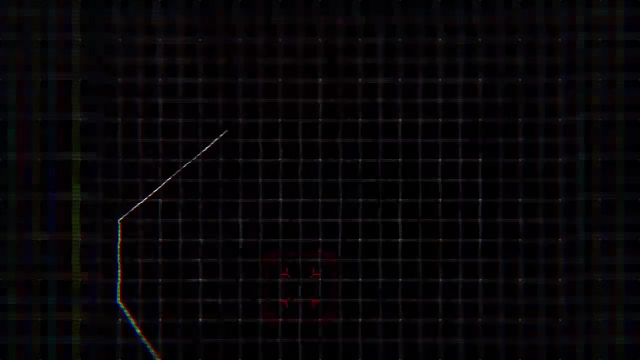 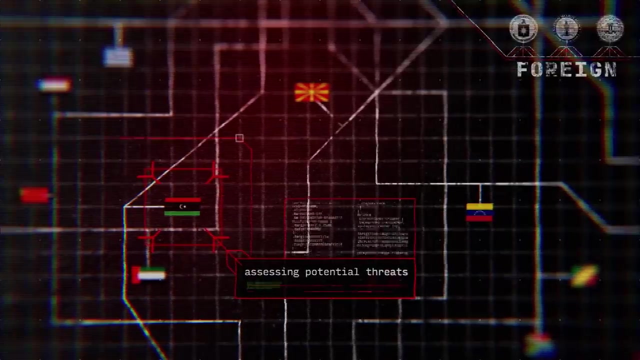 the date, which is a much different thing than the actual content, and the government has very different sets of rules and requirements for obtaining the metadata versus the content. FISA collected information has been at the heart of stopping a number of would-be terrorist attacks. It has been critical. 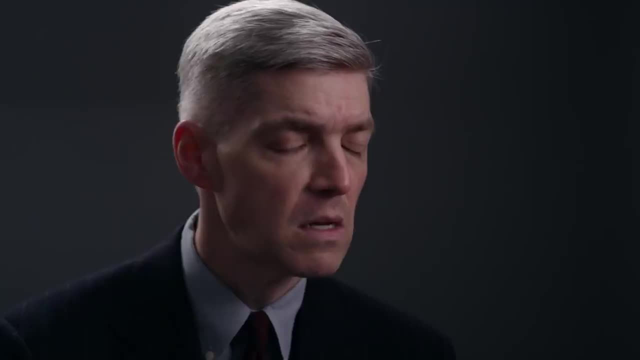 to thwarting a number of attacks that would have killed many Americans. FISA surveillance information has allowed us to uncover a number of espionage issues- So many of the classic espionage folks that have been arrested over the last 30 years that happened because of information that was derived. 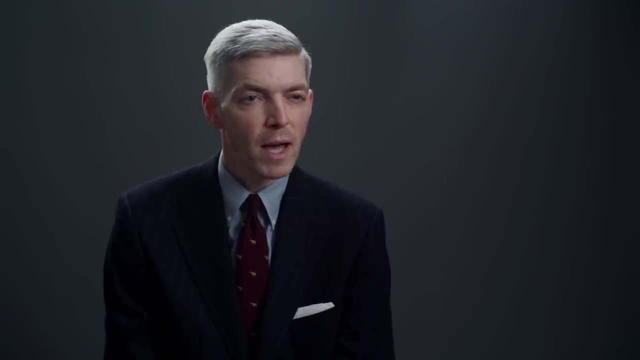 through FISA surveillance authorities. What I worry about is, if we veer too far in the direction of constricting the use of these tools, two things can happen. The first is we miss things. We simply miss information. The second thing is that it could have a chilling effect. In other words, if you make 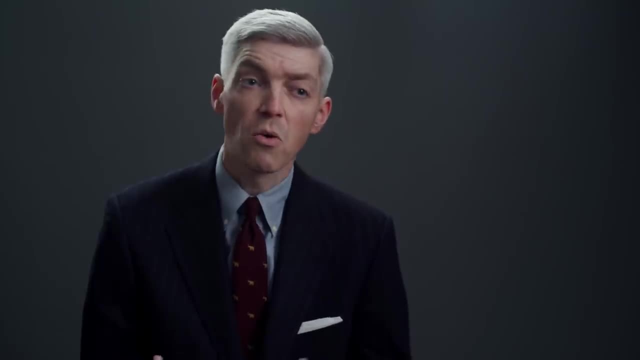 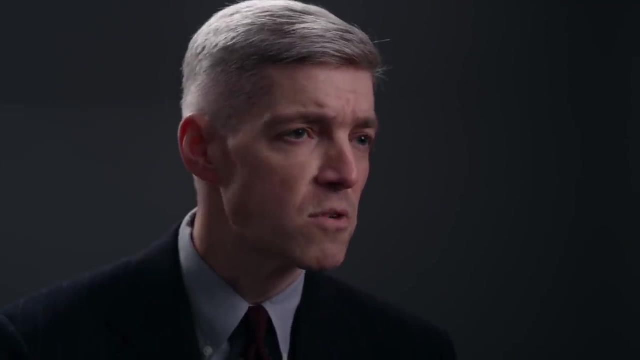 the process so complicated, so difficult, so onerous for an intelligence agency to obtain the authority to run the surveillance. being human nature, many folks will say it's not worth the effort. Even if I could get the authority, I'm not going to fool with it because 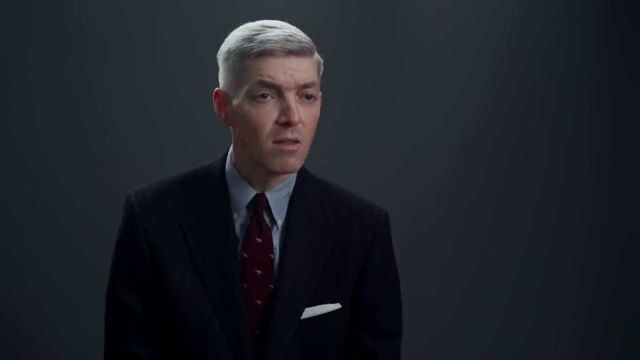 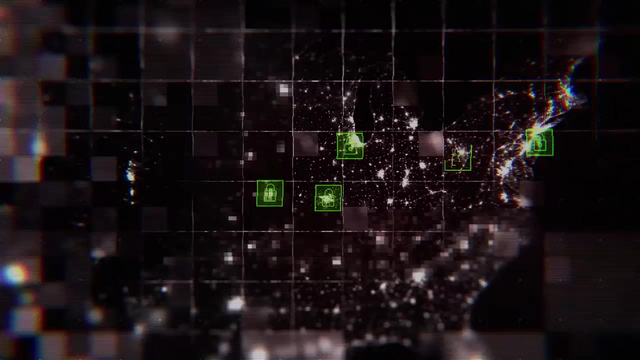 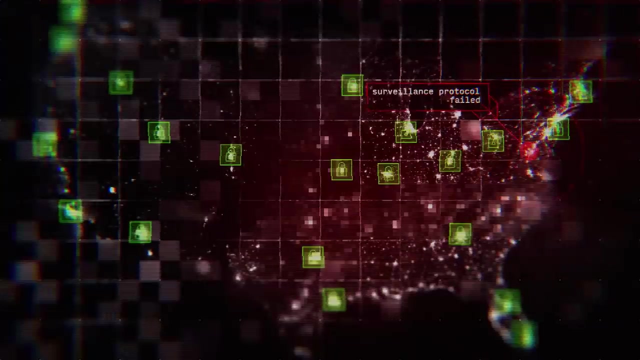 it's too darn complicated, It's too cumbersome, And so, then again, we're missing critical information. We're missing the information we might need for either preventing terrorism, for detecting espionage or for other foreign intelligence needs that the country has. When you're conducting surveillance of a target, whether it's in the criminal context or it's.